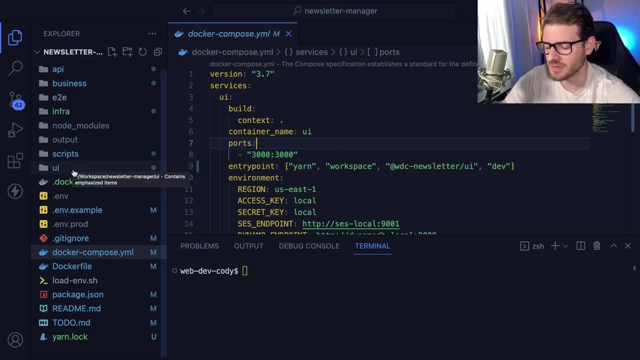 that something is going to break on their machine because they installed the wrong version of a database or they have the wrong version of node, and you end up spending like the whole day trying to help this person out And you realize: oh, you're just on the wrong version of node. 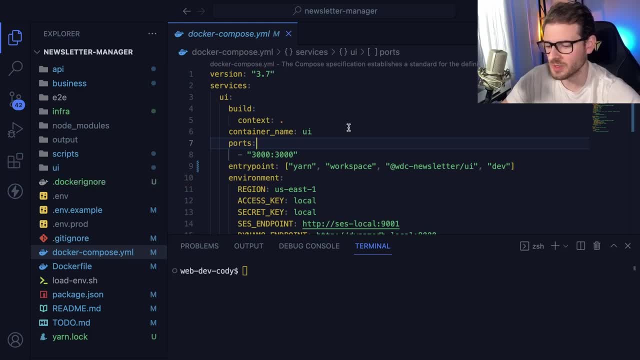 If we just had a way to make this all consistent for all of our 10 or 20 developers on our project, you know this wouldn't be an issue. So that's one aspect of Docker. You can also use Docker to, you know, containerize and deploy your services. 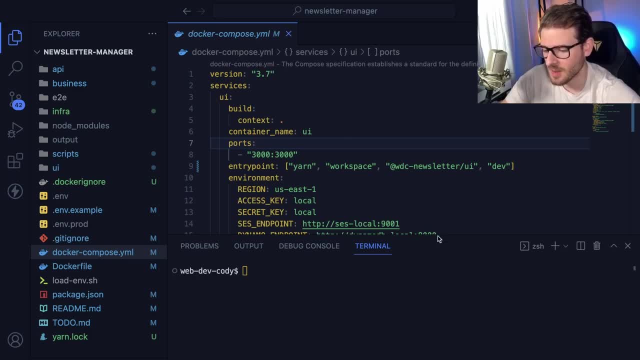 I'm not going to really talk about that in this video. because I'm not doing that in this video. I'm basically just using a Docker compose file so that any developer can clone my repo and with one button they can basically get the entire application running. 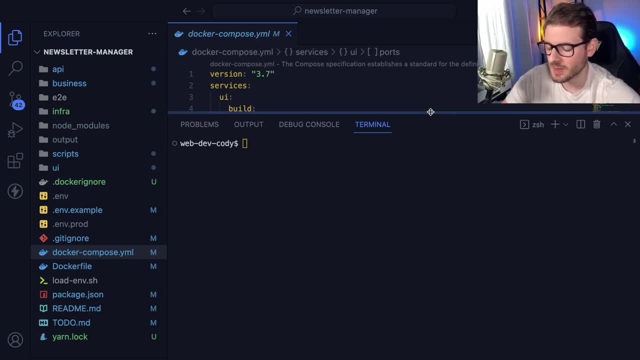 They don't have to read through a readme that has 30 or 40 steps that says, okay, now you have to install MongoDB, Now you have to install DynamoDB local, Now you got to install SES local and then they have to be on a certain version. 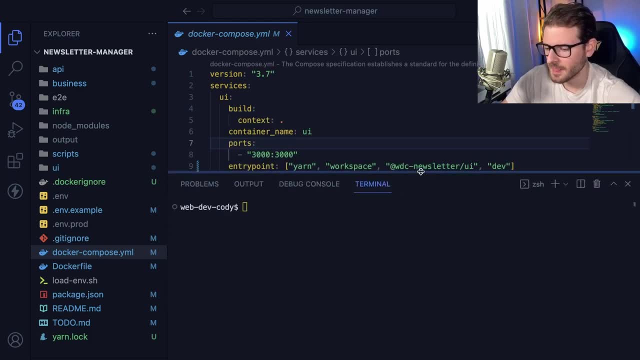 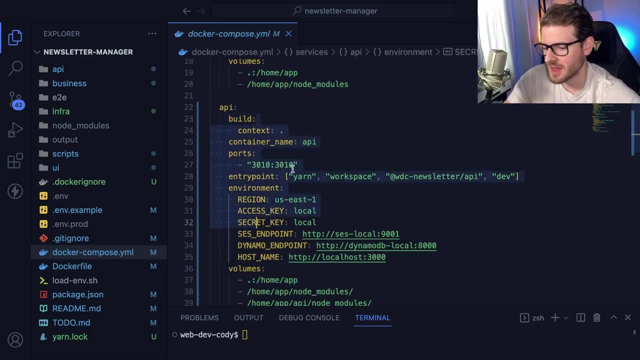 There's none of that right, It's pretty straightforward. So let me just kind of show you the magic real quick. I have a service here that has a UI written in Next, has an API written in Express. It has a local DynamoDB instance, so I can actually store stuff into a database. 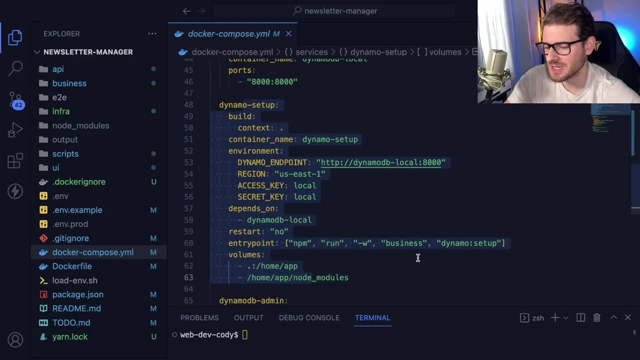 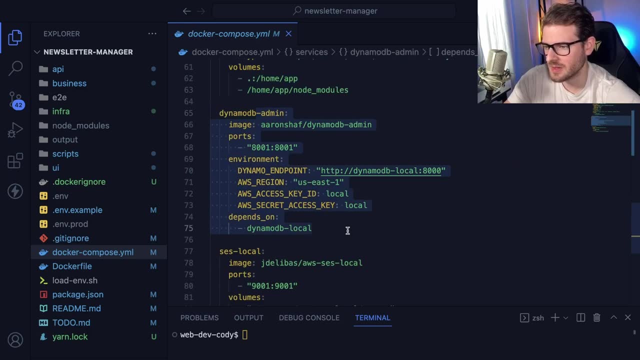 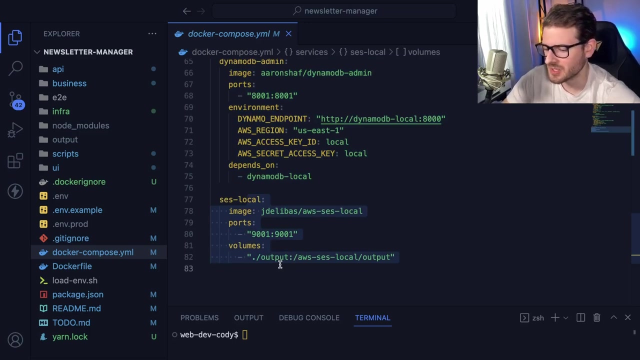 It has some way or some script you have to run to basically inject some seed data into that. We have an admin dashboard panel where I can actually view the database and I also have a local running SES mock service so I can see when emails are potentially getting sent. 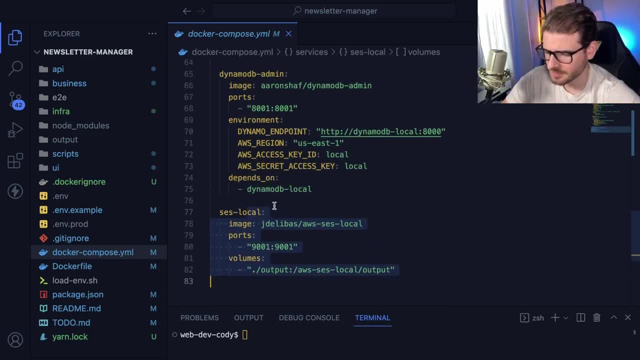 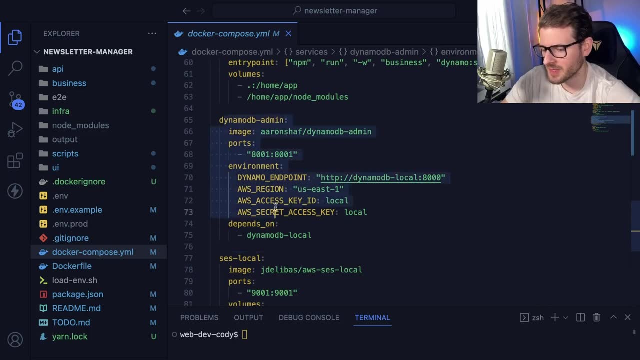 out. That's a lot of things. If you imagine coming into this project as a beginner and having to NPM run this and then load up another terminal and NPM run this one and load up another terminal and do it for this one and that one and that one. it's a lot of extra steps and then you have 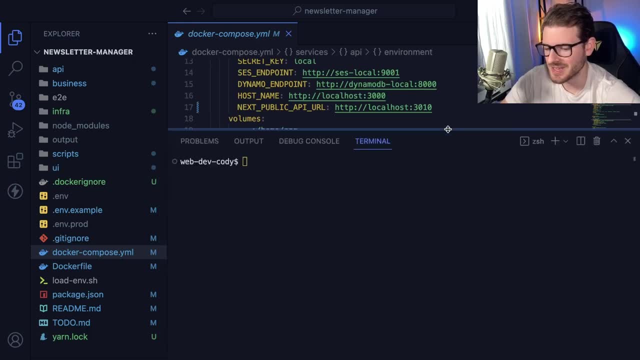 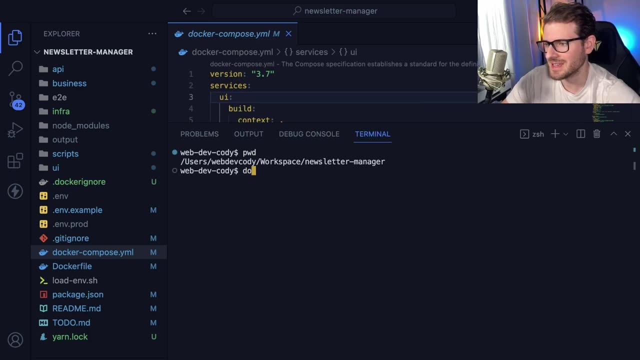 to make sure that every developer has The proper versions, which it's just not going to work right. So Docker is great, because what a developer can do who joins this project is they can say Docker, compose up, and keeping my fingers crossed. I didn't break anything before I. 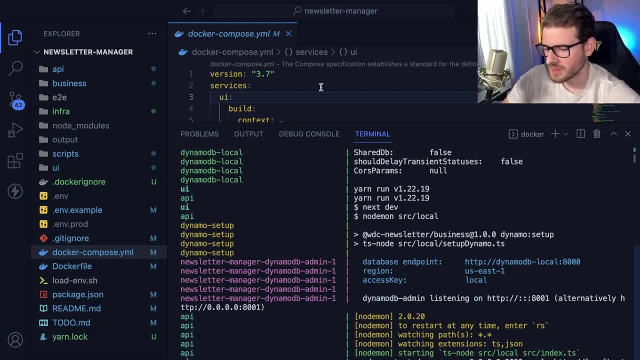 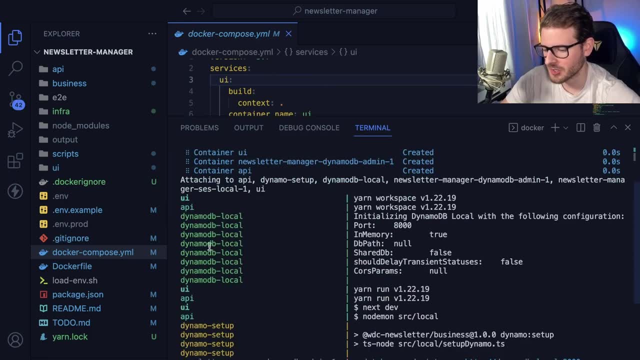 made this video. This is actually going to spin through all of these different services I have laid out in this Docker compose file and that's going to basically run them right. So you can see, here on the left we have different colors of the services. 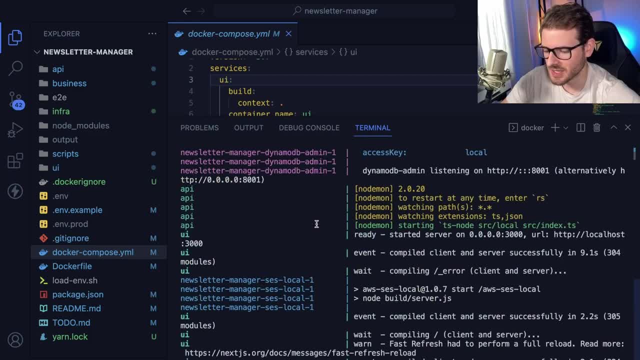 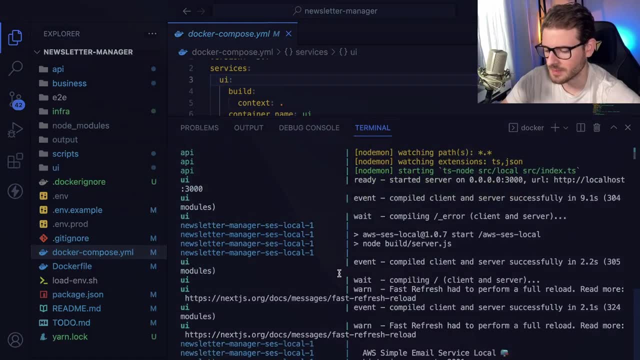 We have UI API, DynamoDB, local. They're all initializing, They're all getting set up and at some point they should be done initializing and I can actually go to my application. So let's just go ahead and go to localhost 3000.. 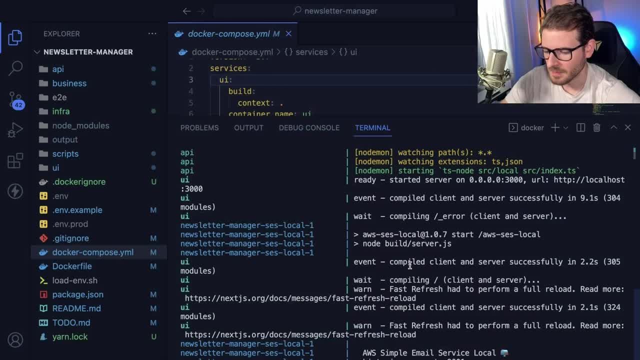 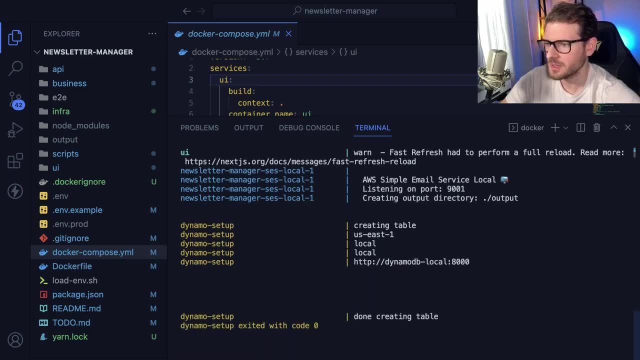 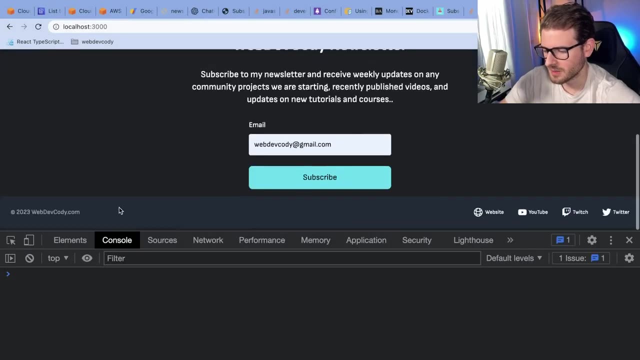 This should be kind of finished running soon. There you have it. The entire application is set up. We have the DynamoDB finished creating tables and I think at this point we should be good to actually use the app. So if I were to go here and just go ahead and say WebDevCody and go ahead and click, 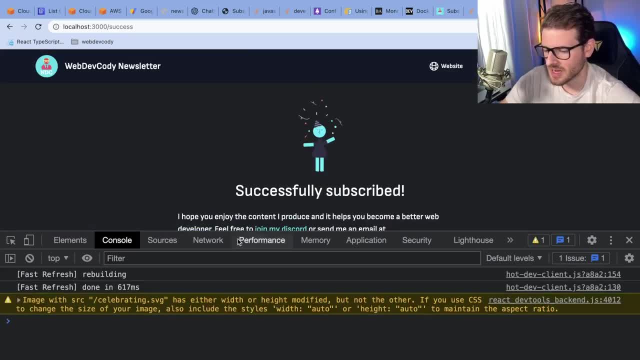 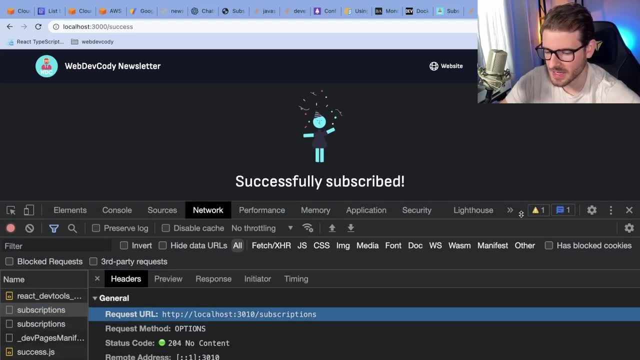 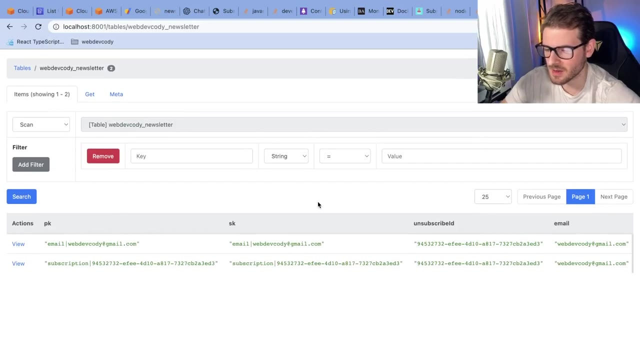 subscribe. Notice that everything works fine. It's actually doing a request to localhost 310,, which is where my API is. That's hitting a database. There is a little web UI running where I can view my database and view the data and all. 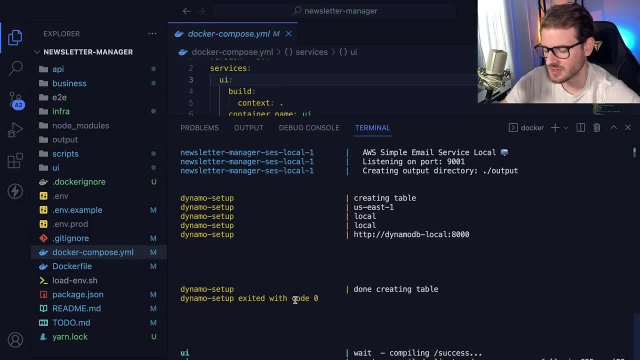 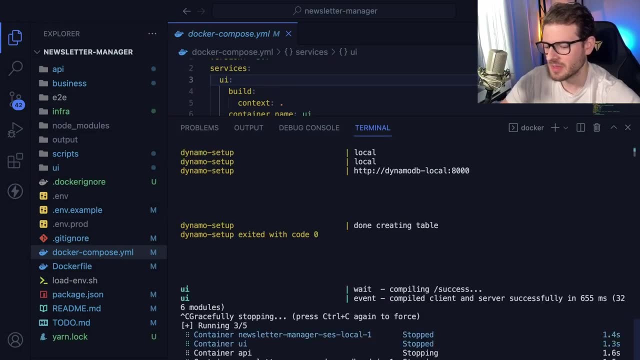 this stuff was set up with literally one command. You guys just watched me do this. I literally typed one command and it spun everything up. and then also, if I command C, it'll spin everything down. right, It'll stop running those services. 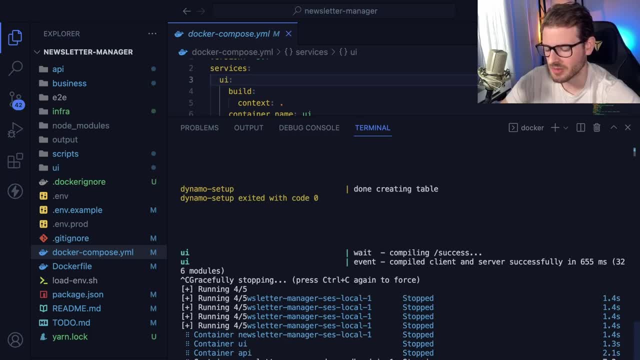 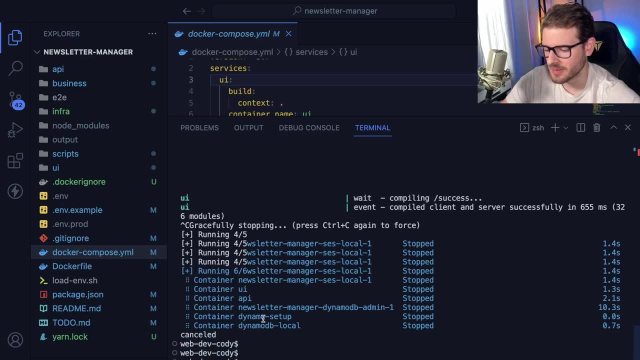 It's going to spin everything down. It takes like five to ten seconds for my application to turn everything off, but all that stuff is contained inside of running Docker images and I don't have to worry about a lot of stuff, right? A lot of the stuff is abstracted away and it's very easy for anyone to just clone this. 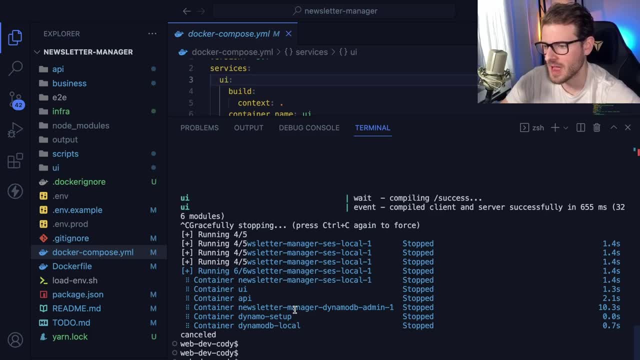 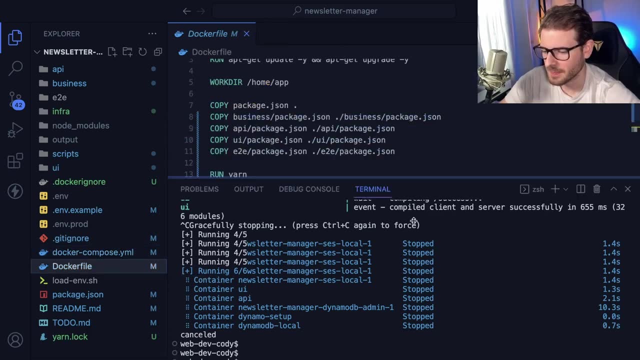 repo, run one command and be able to hit the ground running with adding in some new features. So the gist of this. let's kind of give you a quick walkthrough of how do you do this, How do you set this up. So the first thing I did- 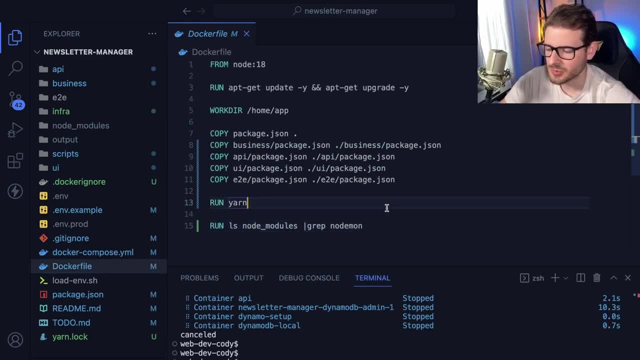 And again I'm trying to figure out. this is even the best way to do it. I'm still trying to learn Yarn workspaces a little bit, so I might not be doing everything proper, But all I'm doing is you declare something called a Docker file which describes your 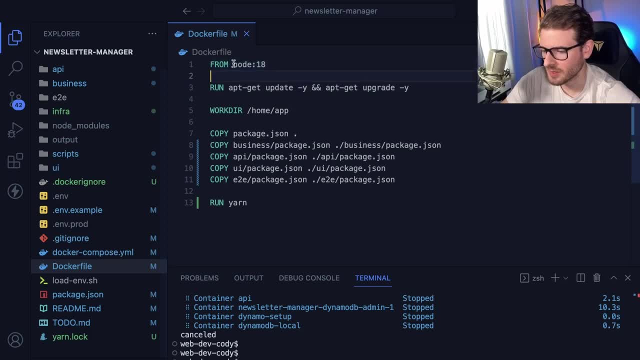 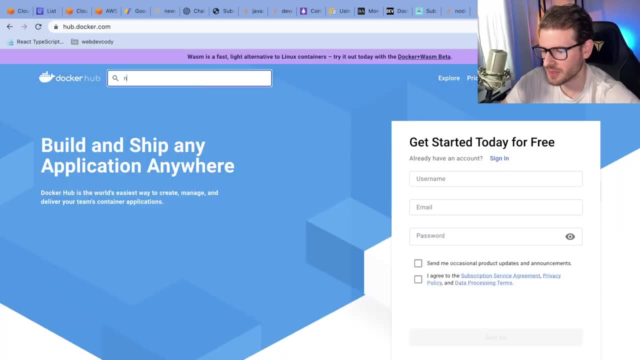 image right. What operating system and what version of Node do you want? Now, if you look at this, this says Node 18.. There's actually something called Docker Hub where you can go and you can search for different Docker containers, right? 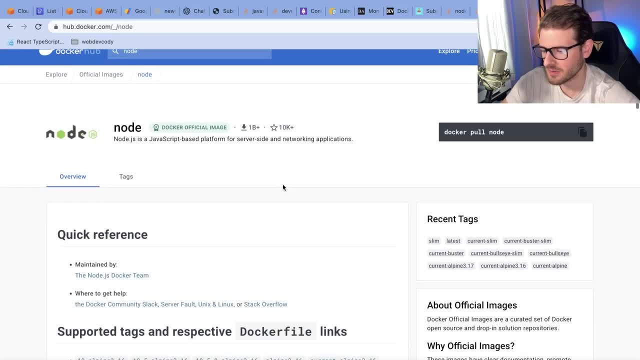 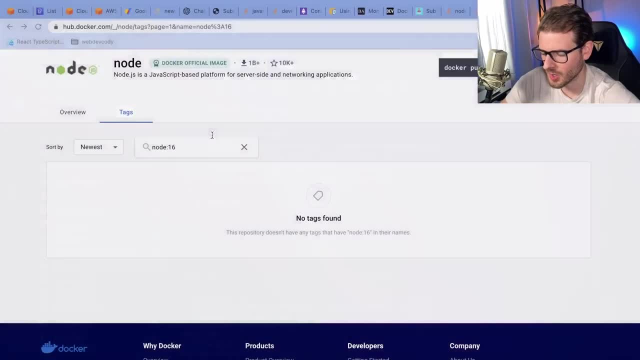 So in this case there's one already called Node right here and if you go and look through the tags, You'll see that there's one called Node 16 or 18.. Let me just type 18.. Let's see, So I can use any of these tags. 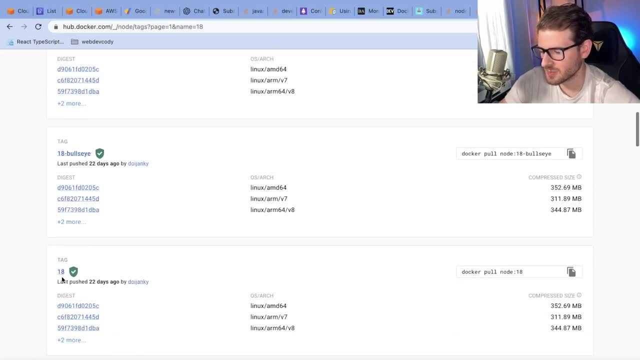 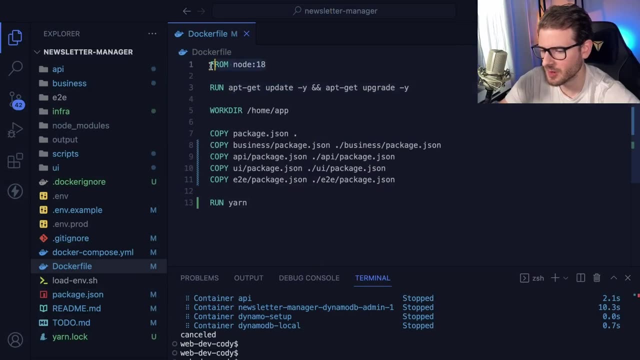 I could potentially say 18.13.0.. I could have potentially just put 18,, which is what I did, And you could see an example over here. It says Node, pull 18.. So this is what the from thing does. 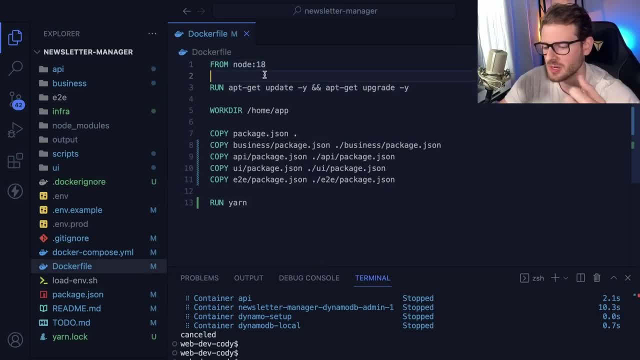 Basically it means go to the Internet, download this container and use that as my starting point And then you can start running some additional commands. So if you're kind of familiar, Okay, With Bash or you know dealing with like Linux and the command line, you can start. 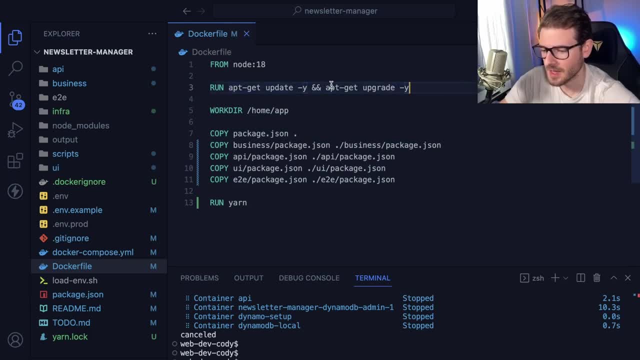 running different shell commands to update the machine and upgrade the packages on the machine, And then what you could do is you can specify inside the image itself what directory do we want to start doing stuff right? In our case, we're saying: go to the home slash app. 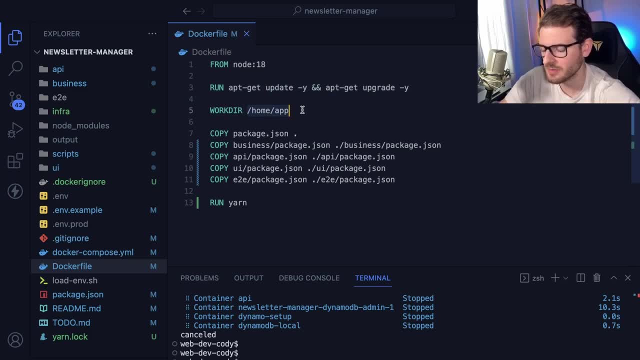 That's going to be our like current working directory where all of our code is going to live, And we're going to copy over some files from this directory. I'm currently in Right. So this copy command basically looks at your files here and it's going to copy from your. 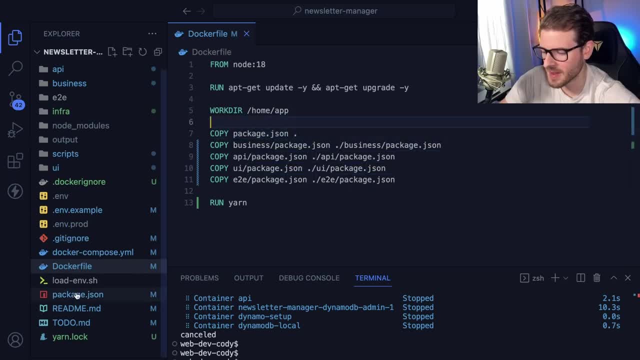 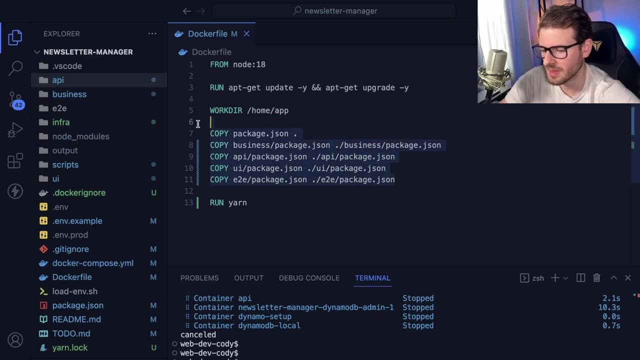 host into the container. So in our case we're saying: copy the package Jason from here, copy the package Jason from business, from API, copy all of these workspaces packages and put them in the corresponding locations And then I'm going to run a yarn inside the container itself. 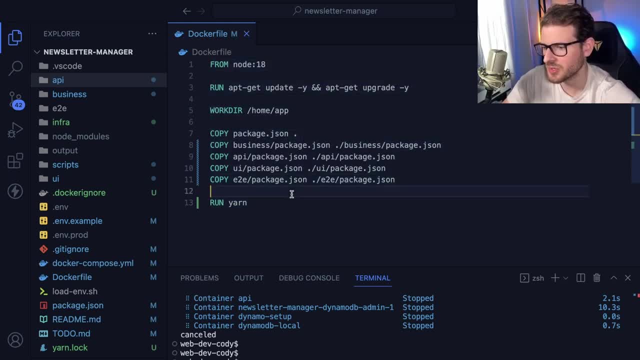 Okay, So this will take like a minute to run. It's installs all the node modules, sets up the workspaces, simple links, sim links and then. So what do we do from here? Right, We have this, this image. we just built a Docker image that has all of our node modules. 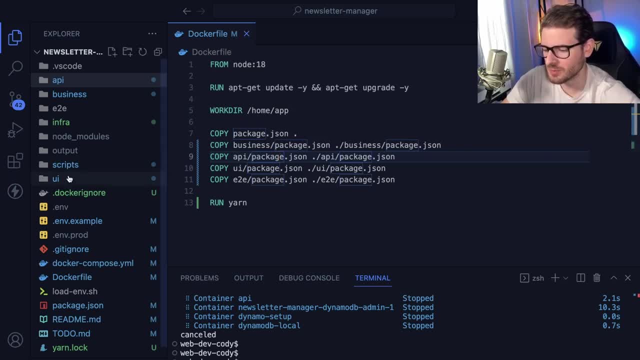 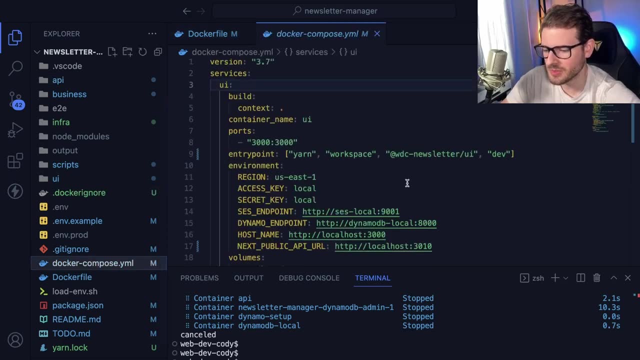 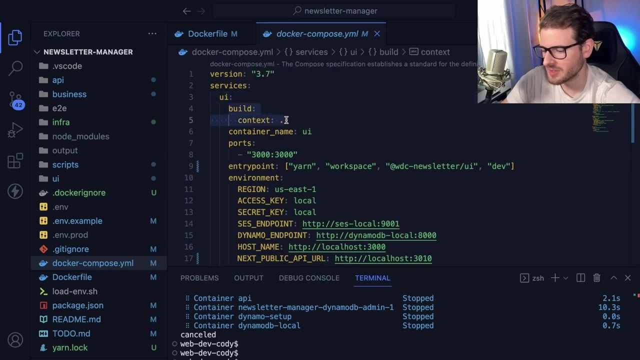 set up, but it doesn't have any of our code in it. Right, It's just a kind of a skeleton project with a bunch of node, module folders and package Jason's. Well, the next step is inside a Docker compose. You can start defining some services and you can say: okay, I want to use the build context. 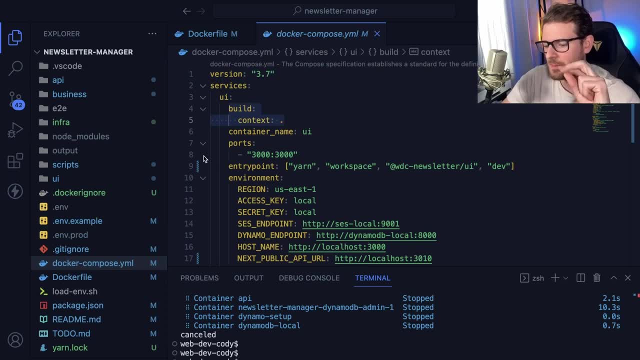 which basically means everything in this directory. I want to kind of Mount everything in this directory And link it inside of that image that we just set up, So it kind of like does a merge between all the existing node modules that are in the box and 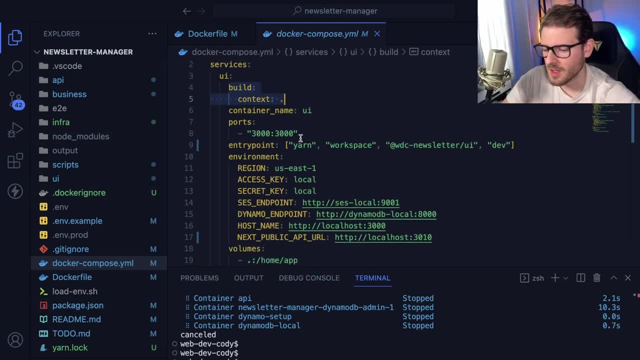 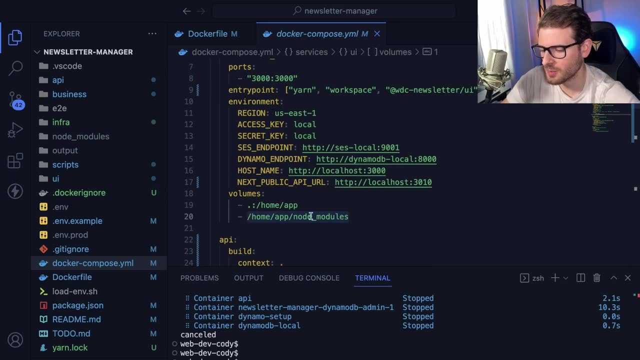 everything that's currently in this directory, Right, Um, but there are some caveats. I basically have to tell it to ignore some files, Like I don't want it to bring over the node modules that are in the top level directory of the host. 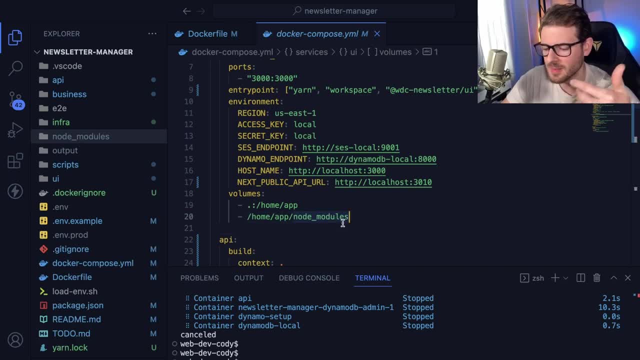 machine because if I do, the host machine might be in windows, it might be in Linux, might be a Mac And I don't want those binaries that were potentially built with like node GYP to overwrite the binaries that were built inside of this um node 18 container, which I 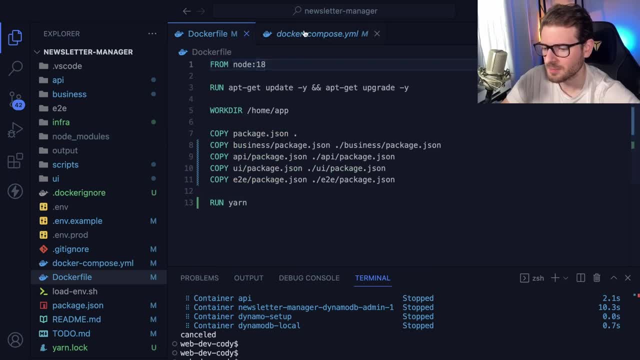 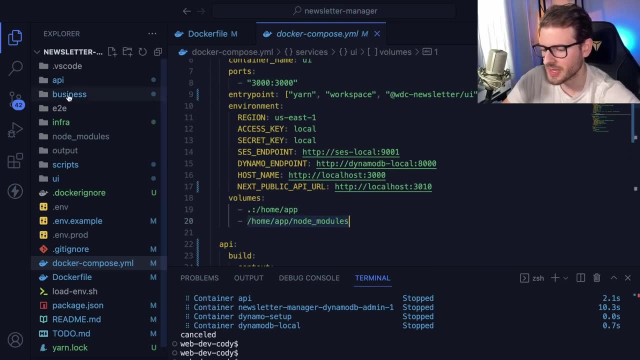 don't know what this is. It might be bullseye, It might be Debbie, and it might be in Boon too, I don't know. but the binaries might mismatch, And this is why I'm saying, okay, I do not want to pull over the node modules that are in the host. 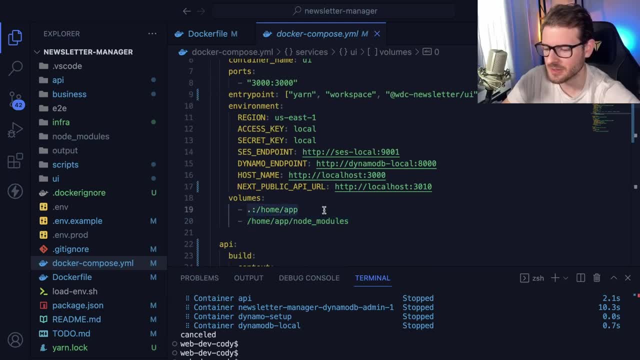 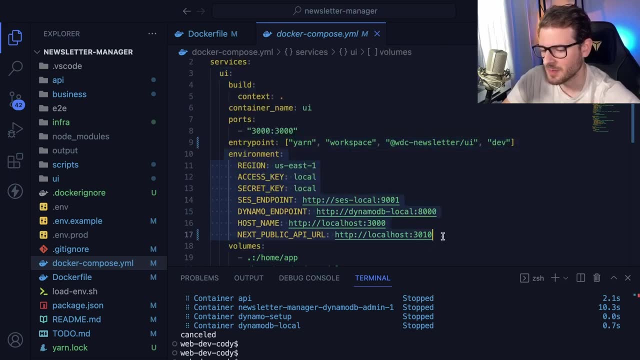 machine, but I do want to pull over every other file that exists on this host machine. So that's what this is doing. It sets up like a, a, a service and I. you know you can specify some environment variables, Like I'm doing here. 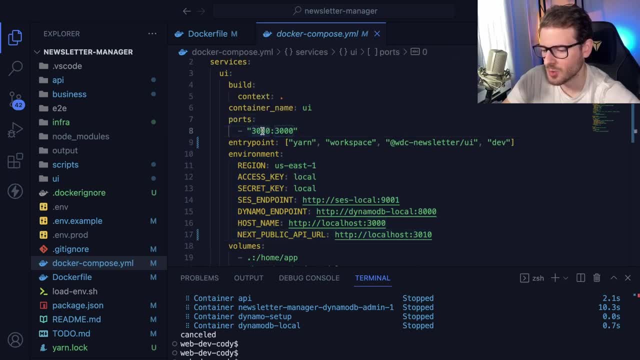 You can specify what We need to map to. this is the host name port and this is the inside the container port. So, for example, if the UI is running on port 5,000, but I wanted to be able to go to port you know. 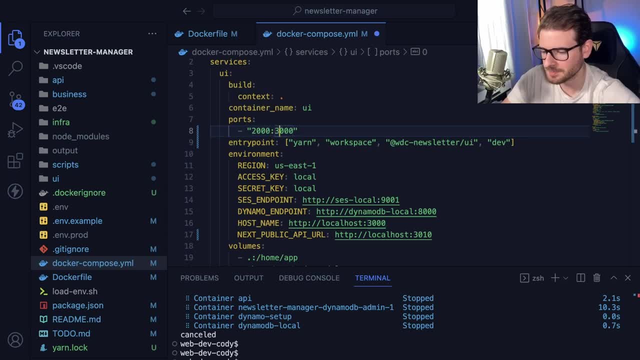 local host 2000. on my laptop I could do that All right. So inside the container you might have next running on port 5,000, but outside of the container you want to hit it at port 3000.. 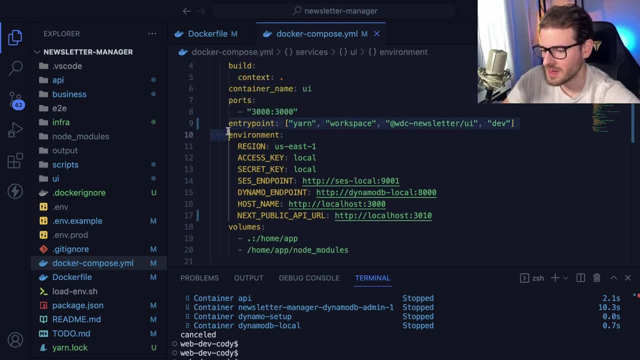 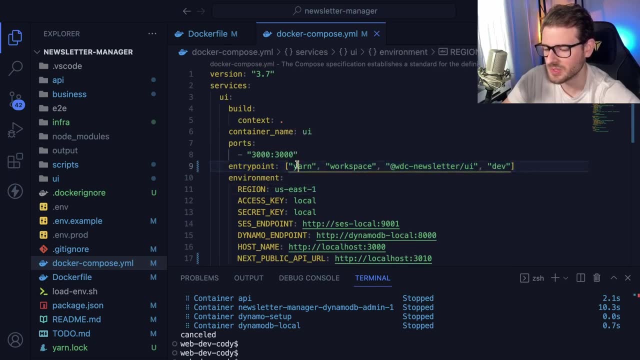 That's just an example. And then the- uh, the meat and potatoes of this is: what do you do when you have this Container set up? Well, you need to be able to run something. And in our case, we're saying: I'm going to do a yarn workspace and I want to go into the UI workspace and I want to run the dev command. 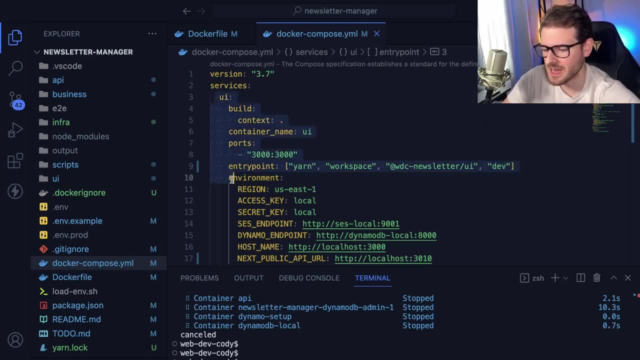 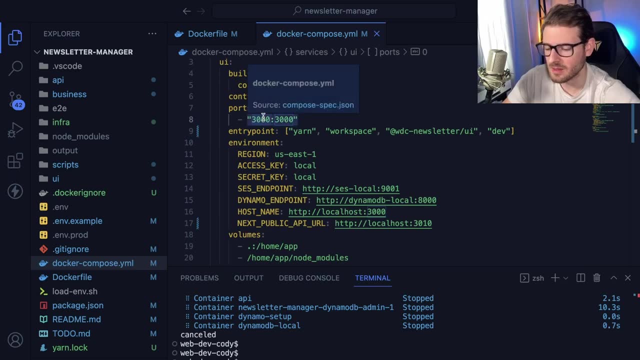 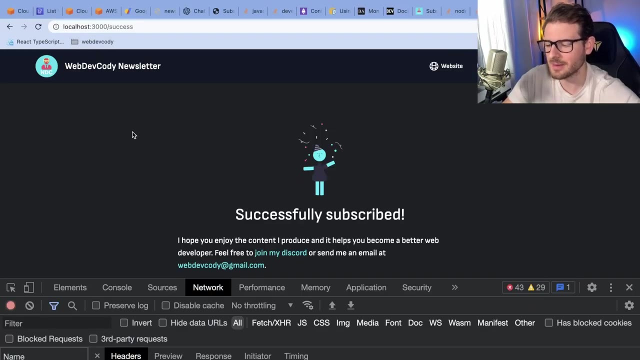 That's going to basically run next inside of this container And it's going to host in a port 3000.. I'm going to map it to 3000 on this host machine And there you have it. You have next running and I can actually access it, which is what you saw earlier when I showed you this. this was the next that's running inside the container. 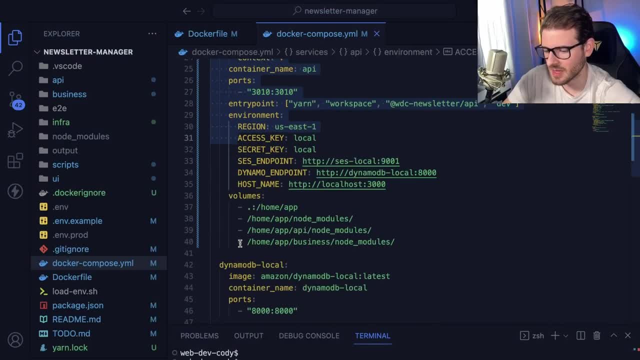 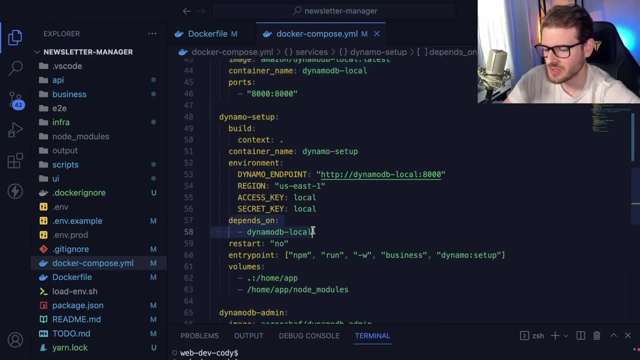 So basically copy and paste what I just said For everything. We do the same thing for the API. We do the same thing for Dynamo, local Dynamo setup. There's one cool thing about Dynamo setup which it's saying it this depends on Dynamo DB local to finish running before you start running the script, right? 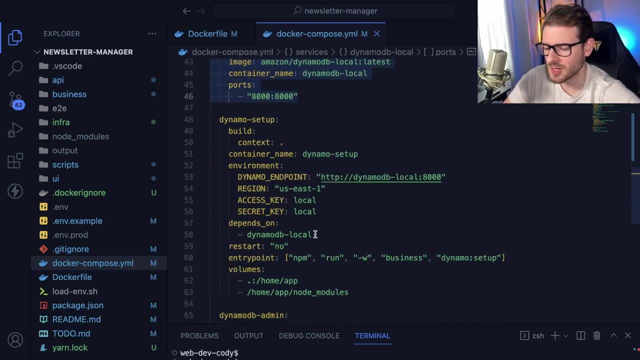 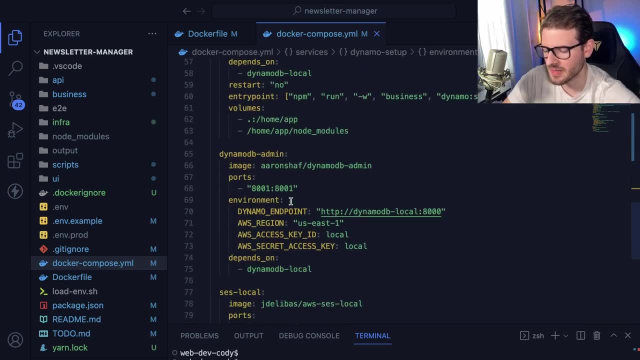 So you need to make sure the database is fully running before you start trying to inject C data. So that's why this depends on. is here There's probably some cleanup I could do with the environment variables and stuff like that. This thing should probably not be an NPM. 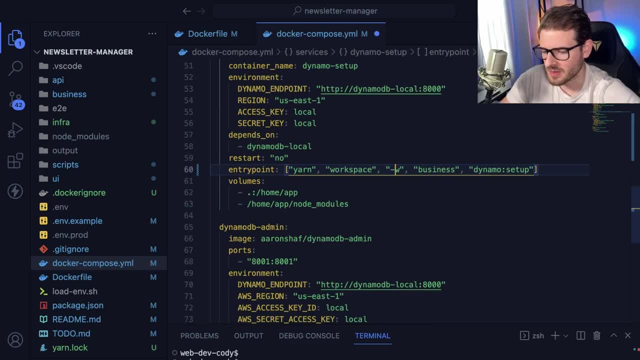 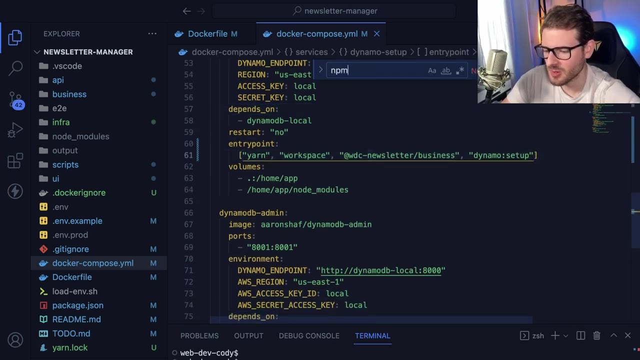 This thing should probably be a yarn workspace, And then I should. I should probably say like: add WDC, um newsletters, slash business. and then I want to go ahead and run Dynamo set up. make sure I don't have NPM anywhere else there. 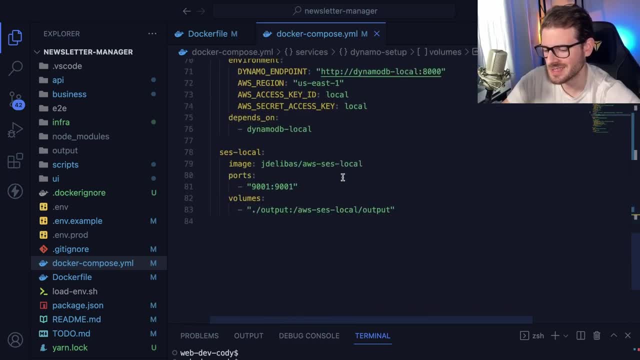 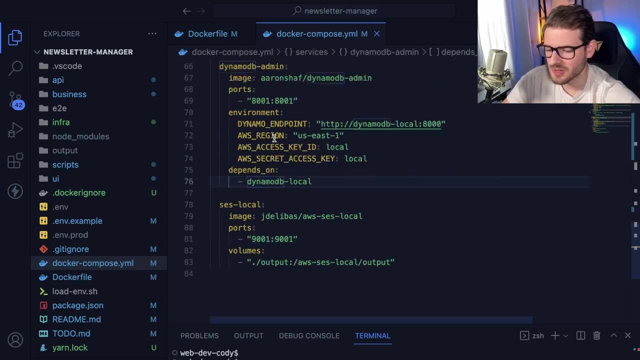 I was originally using NPM workspaces. I decided to refactor the yarn workspaces. It seemed like it's a little bit nicer. It's a nicer developer experience And, um, I'm sure I missed something about Docker. Docker is a very, very complex thing. 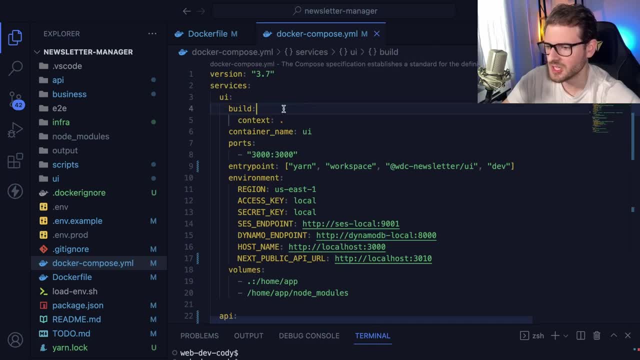 It has a lot of things you can kind of dive into and learn. But I just want to kind of like walk you through some of the things that I'm doing on this project just to kind of get you exposed to Docker If you haven't seen it before and kind of you know, let you know that there's benefits to Docker. 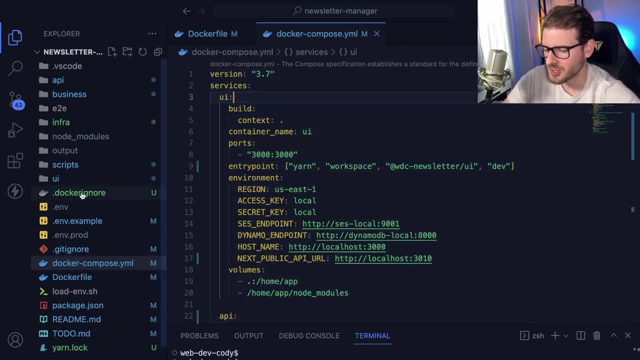 Some people think this is a lot of overhead, but when you get on a larger team, are you? let's say, you work on multiple projects? Let's say you have five or six different clients and they all have different projects: One's in go, one's in Python, one's in- uh, you know JavaScript and no JS. 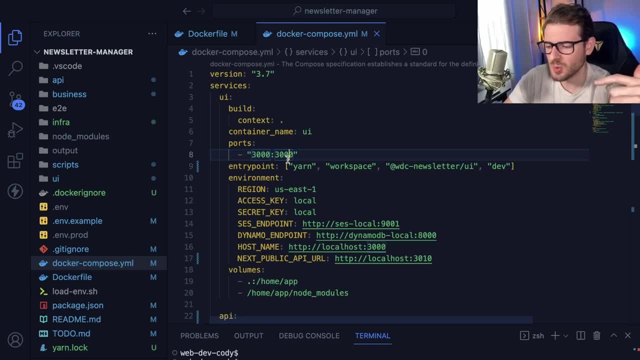 It's very easy: Just CD into your project, do a Docker, compose up, And then everything needed for that project is just set up, right The same like, which is kind of what I showed you at the start of this video, right. 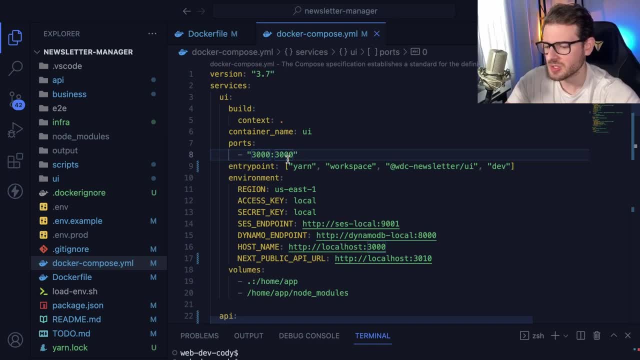 Everything you'd ever need to to work on this project. It's right there. It's all outlined in a Docker compose file and you can hit the ground running just by writing a single command. Well, I hope you guys take some time to look into Docker.